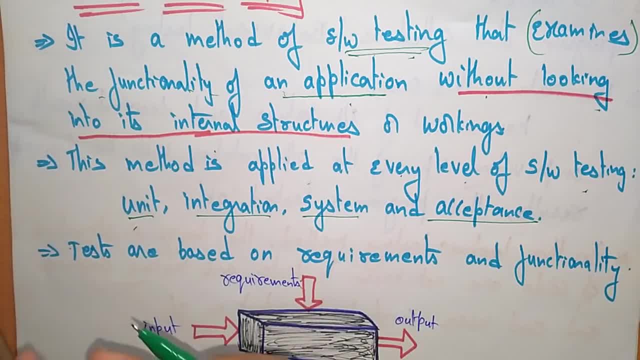 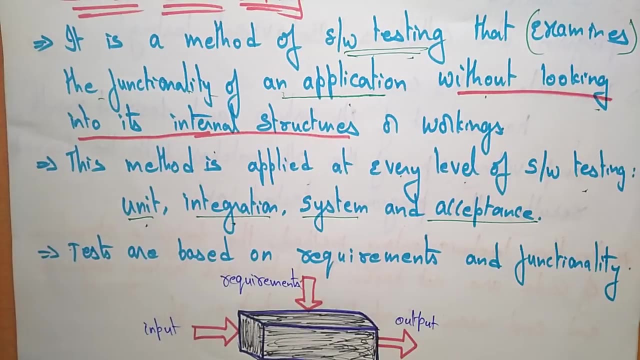 testing. so you may get the doubt. I said black box testing is only examines the functionality of an application. it doesn't look into the internal structure. but it is applied to unit and integration. so the unit and integration testing, everything will be done on the coding. okay, so here the unit testing will be done on the module. 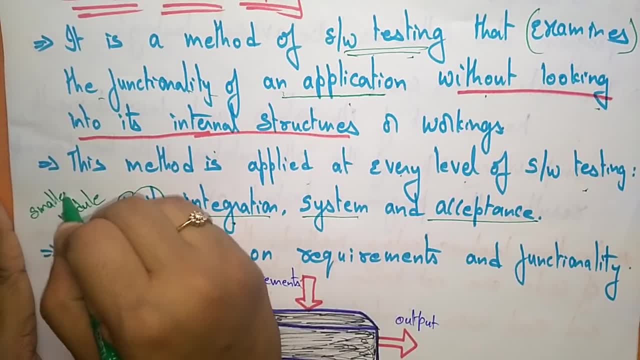 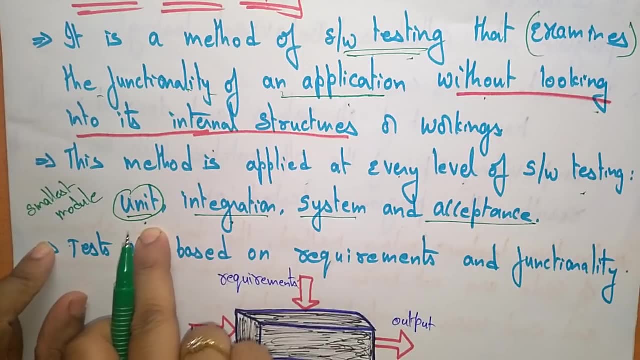 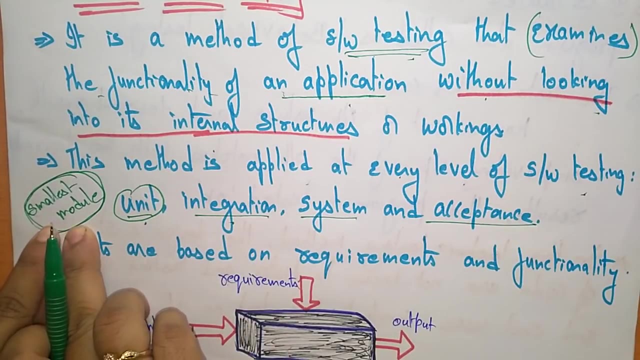 it is the smallest module. you can take it as a smallest module. so inside the smallest module. if you want to test the code, that will be done by unit testing. so the smallest module application. okay, that smallest module. functionality of an application will be tested by the black box in. 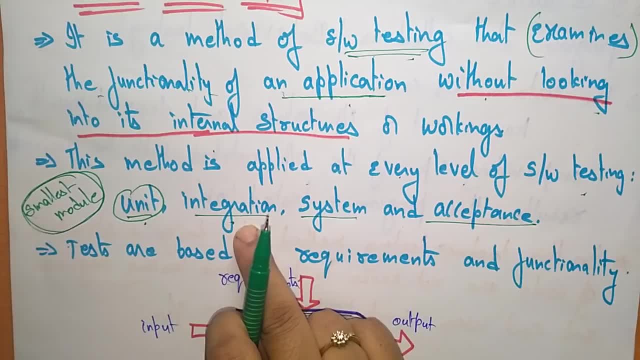 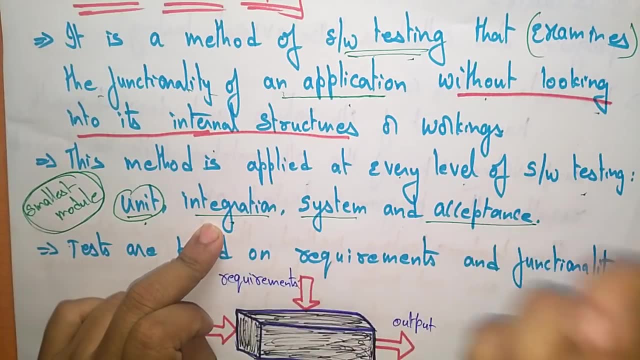 the same way for the integration. whenever you are combining all the smallest element into one element, that there you will done the integration testing. so the integration testing will be in that internally. what is that? how the code is interacting, is able to communicate all the modules. so here the Black Box testing will only examines the functionality of an integration testing examines the functionality of an integration testing application. so in a way system and acceptance. so the testers are based on requirements and functionality. so here the main testers will be based on and functionality. so it doesn't bother about the internal structure and the 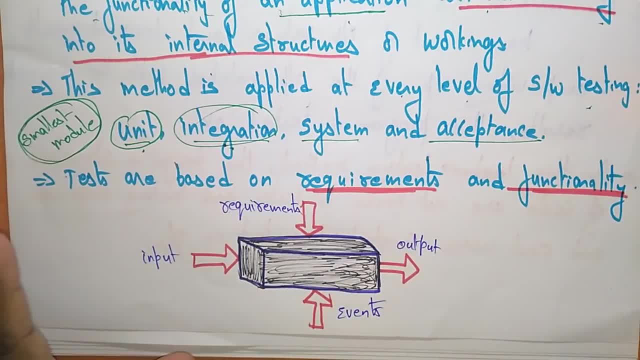 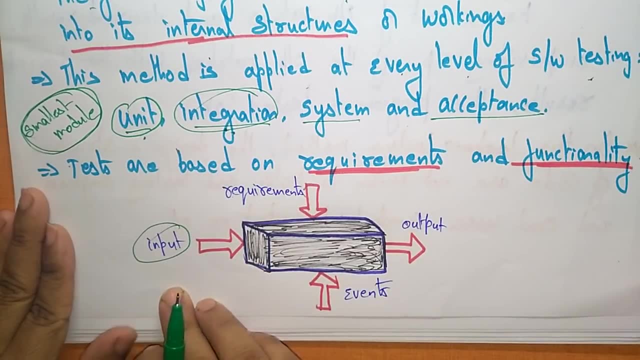 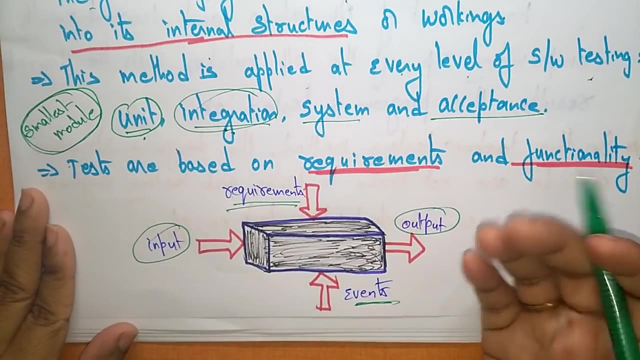 code. it only based on the requirements and functionality means what is the functionality and what is the requirements. now, that is the input, whatever we are given, and the output you are getting and the requirements that we are giving, okay, and the events that are going to be executed. so it is only focus. 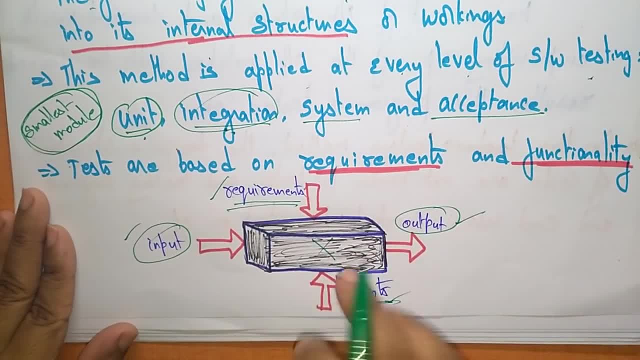 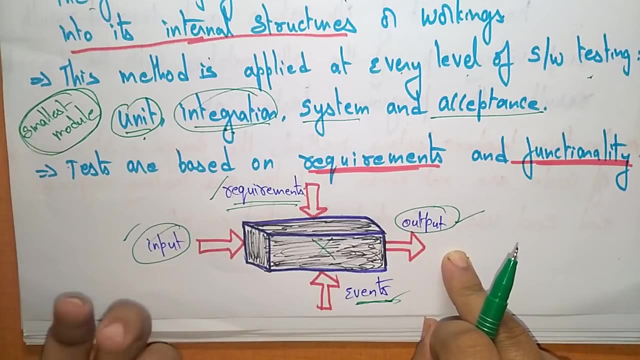 on these elements. it doesn't bother about what is going on inside. so you are going to test what are the inputs that we are giving. is it the correct input? and whatever the input we are giving, the output will getting. what the customer wants means is the math. is it matched to the exact output so that you have to be? 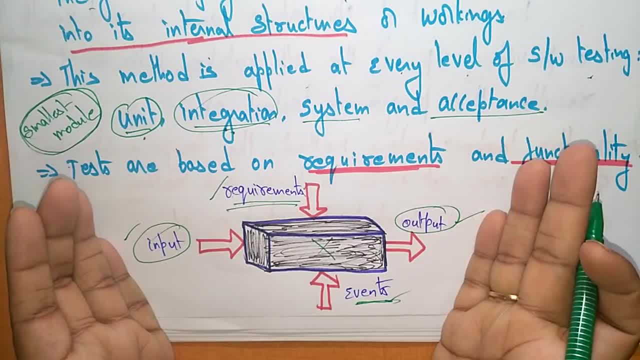 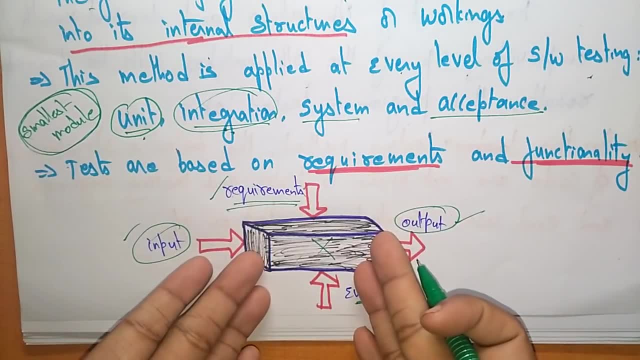 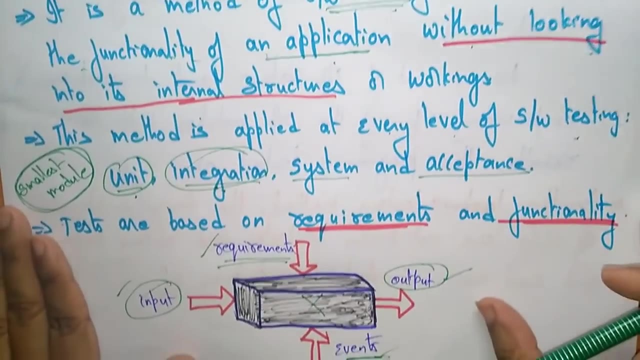 tested based on the input you. are you getting the correct output or not? okay, and the requirements that we are giving is correctly or not, and the events that are going to be executed internally on the on this application is correct or not? so that will be tested by with the help of black box testing. so it is carried out, it is. 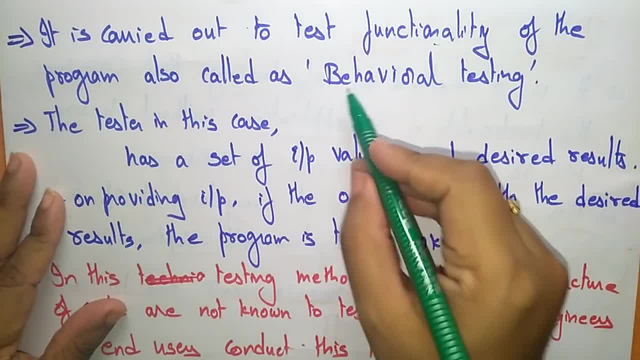 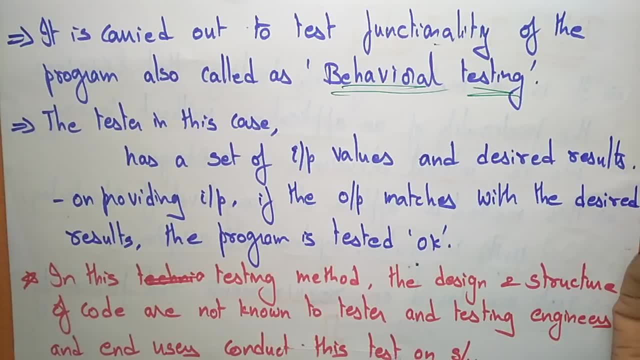 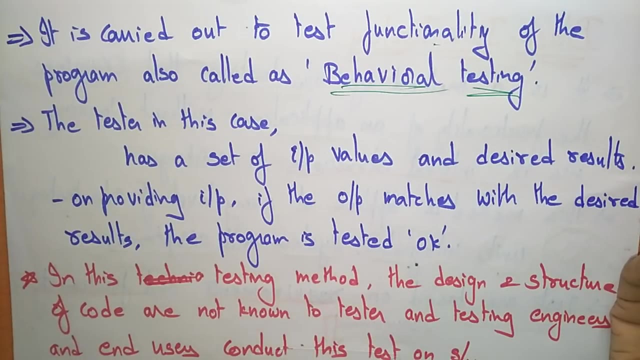 carried out to test functionality of the program and you also call as a behavioral testing- so it is the another name for this black box testing is behavioral testing means it is testing the only on the behavior things like input and output and the requirements and the functionality events like that. so that's why we call it as a behavioral testing. 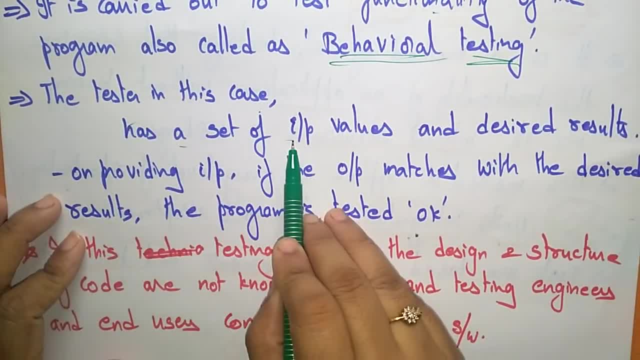 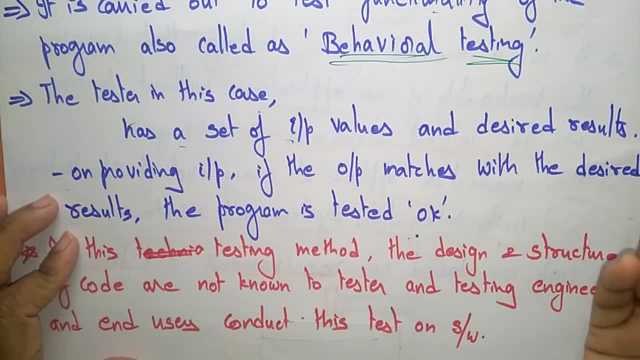 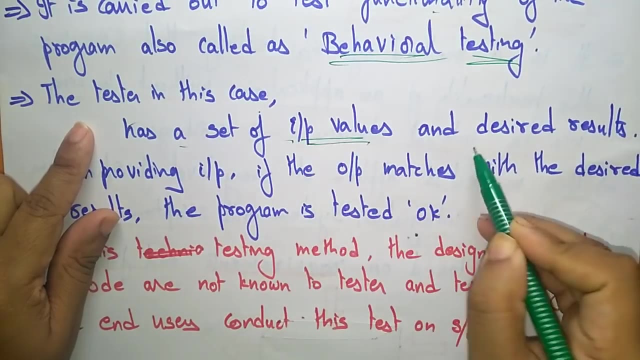 also. so the tester in this case has a set of input values. the tester is nothing, but is a person who is going to be tested, whether it is a customer or whether it is a developer, whatever person he may be. so that person will give the set of input values and the desired results. so first he gives a set of input values and results. 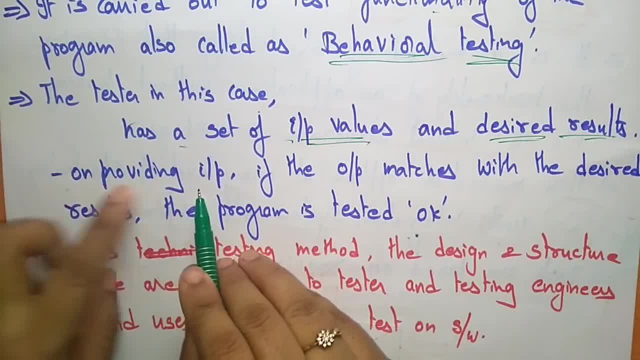 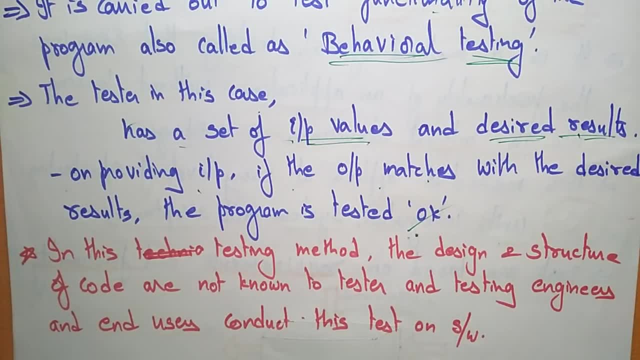 and the desired values for that input values. on providing input: if the output matches with the desired result, the program is tested. okay, so, starting only, we will give the set of input values and for that input values we will get the desired result. so that is the exact procedure. 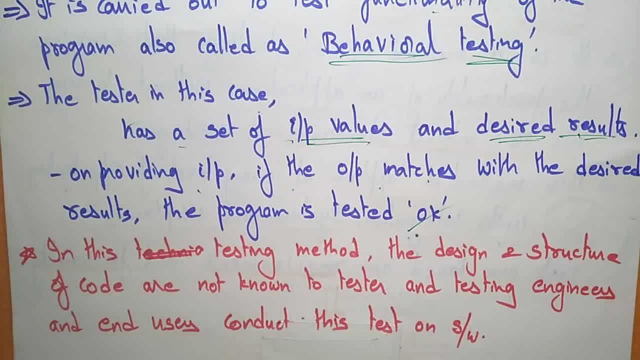 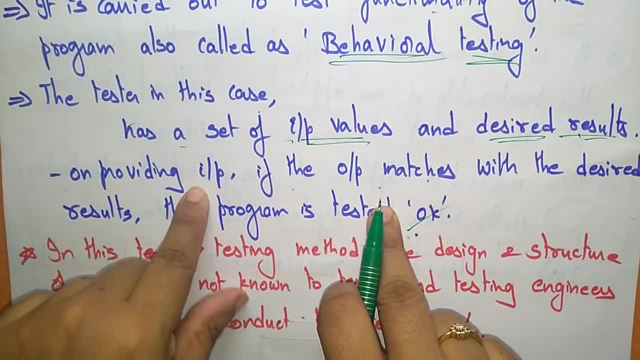 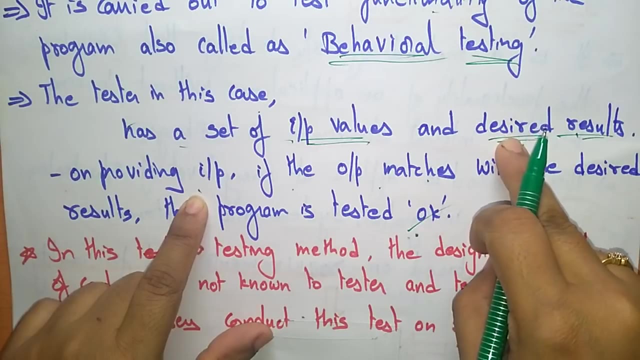 so whenever you are so here, black box testing is going to test first. it is giving one input value and it is matching the output. whatever that we get based on this input, we will meet the requirement of the desired result or not. okay, if it is meet the desired requirement. 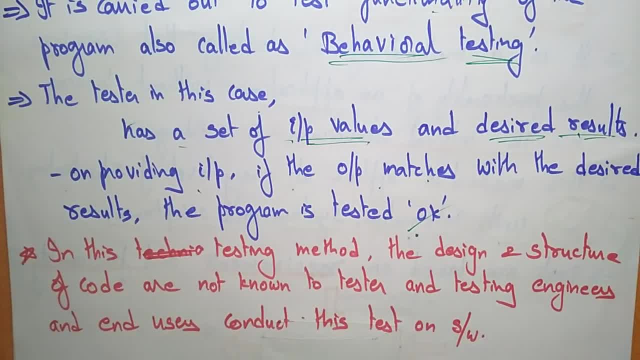 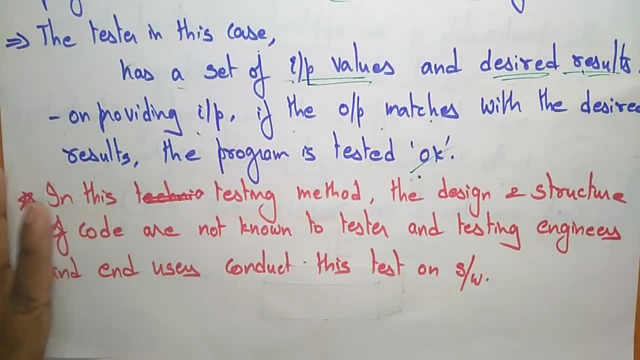 then the program is correct. if the, if it does not meet the requirement, it does not meet the desired result, then the program is having some error. okay, so in the, in that way, the black box testing will be used. in this testing method, the design and structure of code are: 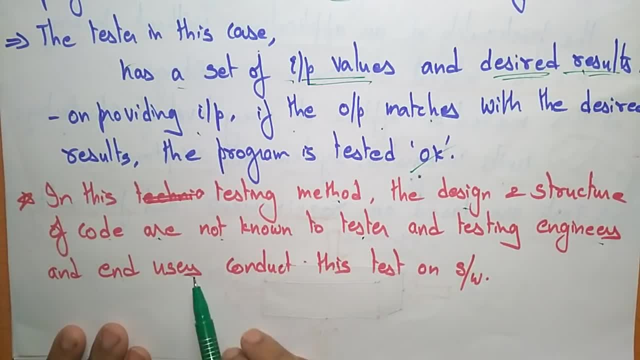 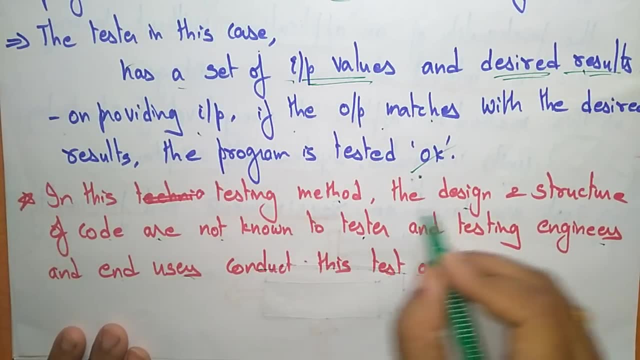 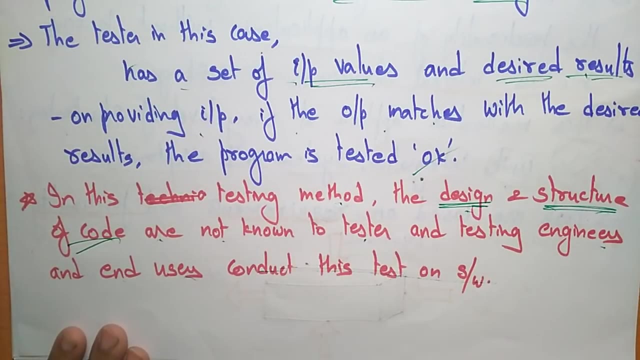 not known to test tester and testing. engineering and end users conduct this test on software. so again, I said that the testing method only concentrate on the design and structure of the code. design and structure of the code. it doesn't bother about what inside the code, okay, what it will be there inside. 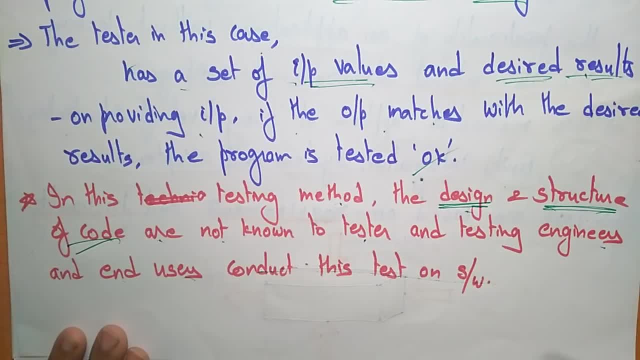 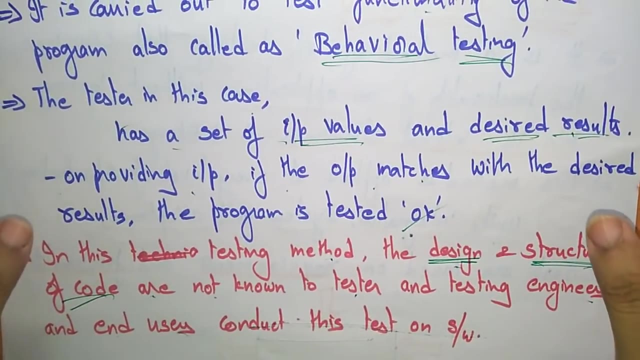 the code and it doesn't test. is there any errors in the inside the code? okay, it's only think about the design and structure of the code are not known to the testers and the testing engineers and end users conduct this test on software, so this is about the black box testing. thank you.